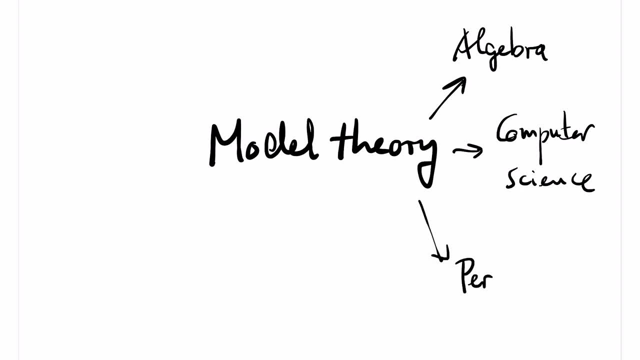 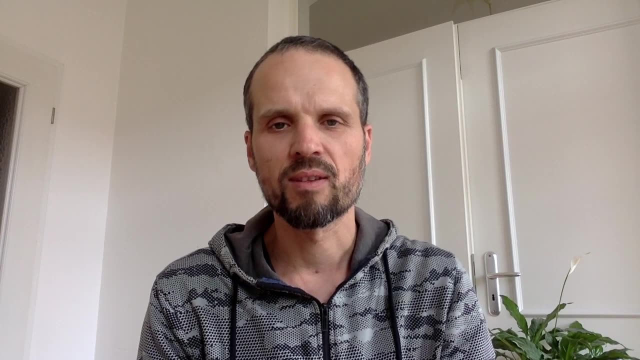 In this course we will also see many links with the theory of infinite permutation groups. Model theory often uses results from combinatorics such as Ramsey's theorem, And for some topics in model theory a bit of set theory is needed. One of the general goals of model theory is to understand 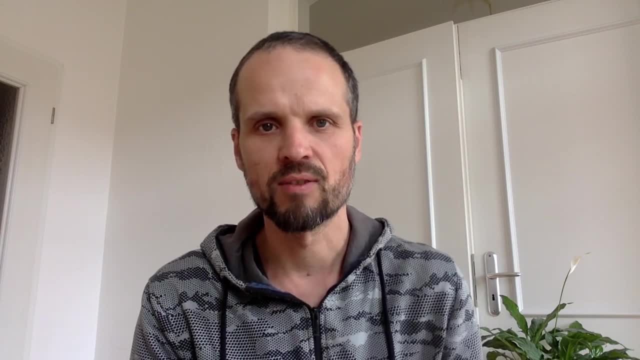 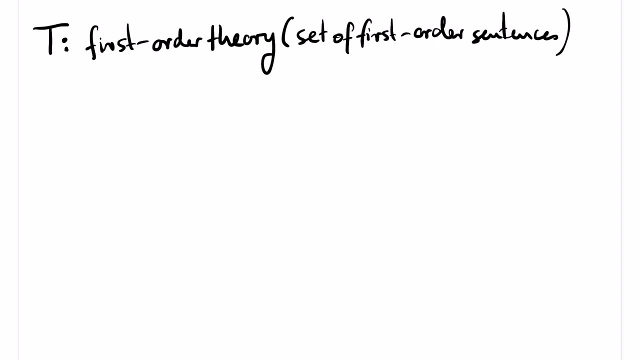 the class of all models of a given first-order theory. t a first-order theory is just a set of first-order sentences, For example the theory of groups, or the theory of rings, or the first-order theory of one of your faces. 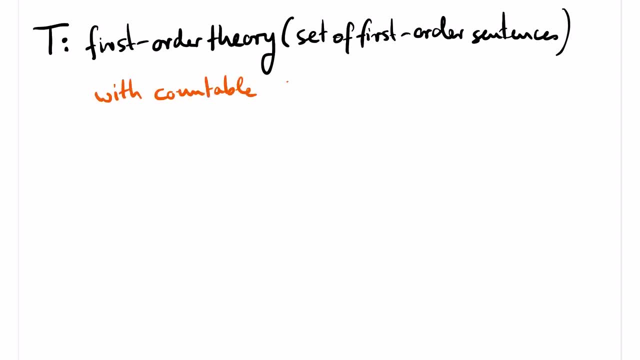 And the theory of the first order, of the second order, of the first order of the first order. For simplicity, I assume throughout the video that t has a countable signature. A concrete and fundamental question that one can ask about the class of all models of t is: 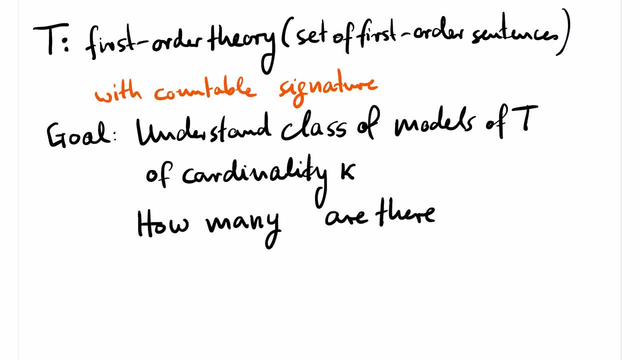 how many models of some fixed cardinality kappa are there? If we count models, of course we actually want to count isomorphism, classes of models, So isomorphic models should only be counted once. For example, if we look at the first-order theory of some finite graph, 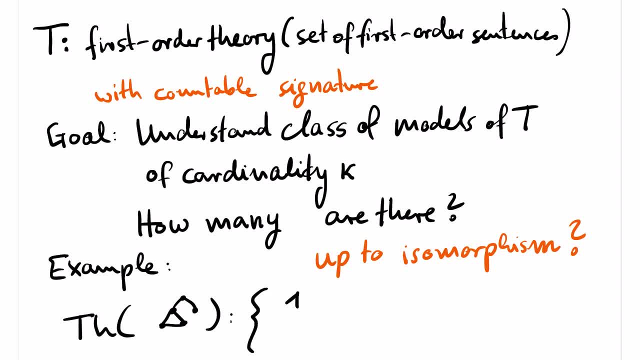 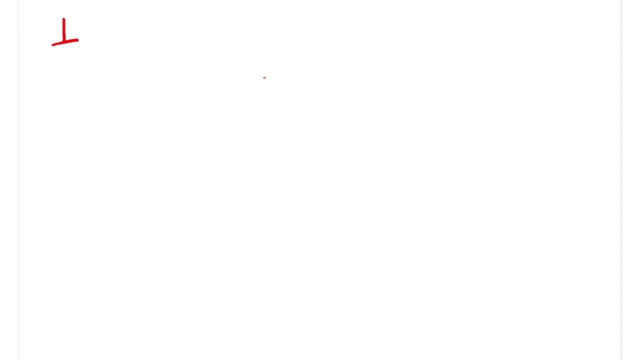 with five vertices here, for example. then there is one model of size five And all other models must be isomorphic to this model, because with first-order sentences we can completely describe the isomorphism type of our finite graph In the following: i t kappa denotes the number of isomorphism types of models of t of cardinality kappa. 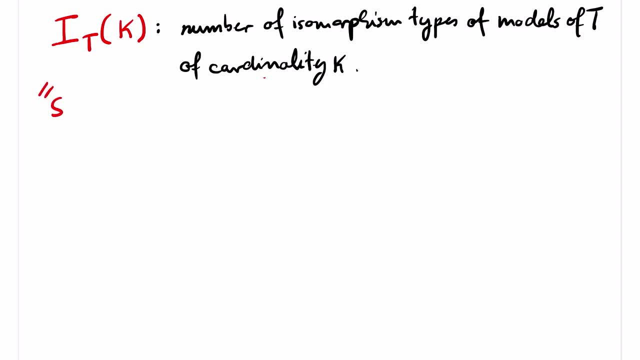 The function is sometimes called the spectrum of t, i, t. kappa is the number of countable models of t. By what we've observed, the number of countable models of the theory of some finite structure, for example, is zero. Now let's have a look at something more interesting. 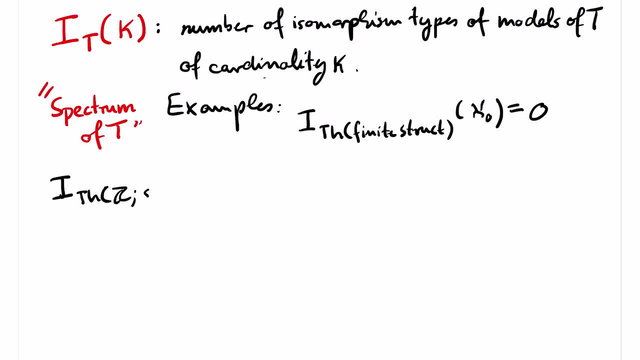 Let's look at the first-order theory of the integers with the successor relation. The first-order theory of this structure contains, for example, the sentence that states that every element has a unique successor, a unique predecessor, By definition. we have at least one countable model of this theory. 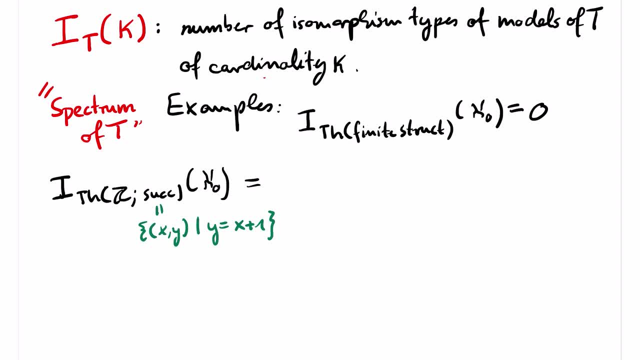 but there are also countable models that are not isomorphic to the model we started with. For example, we can form a disjoint union of two isomorphic copies of the original model. In the resulting structure, it is still true that every element has a unique successor. 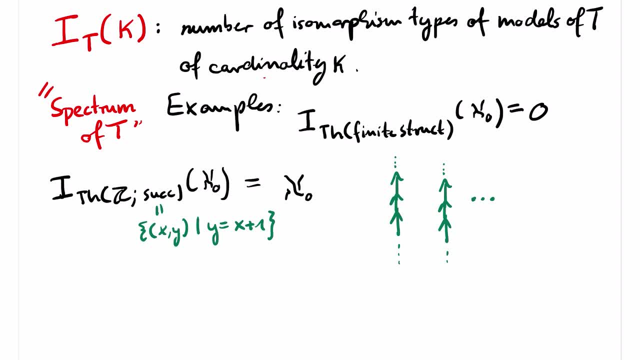 and a unique predecessor, and it is still countable, but clearly the two structures are not isomorphic. To work out the details of all this is a good exercise. My next two examples will be treated explicitly later in the course. I present them here as facts without proofs. The first is that 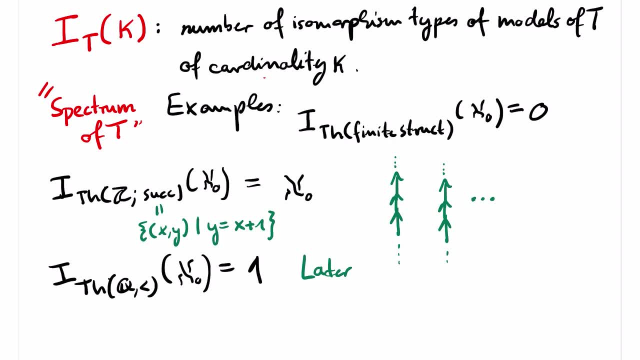 the theory of the order of the rationals has exactly one countable model, So first-order logic describes this structure uniquely, up to isomorphism. The second is the other extreme, the first-order theory of the rational theory. rational numbers with addition and a strict order has continuum many, that is 2 to the. 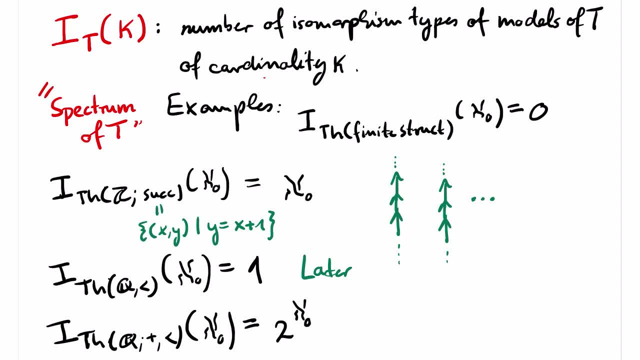 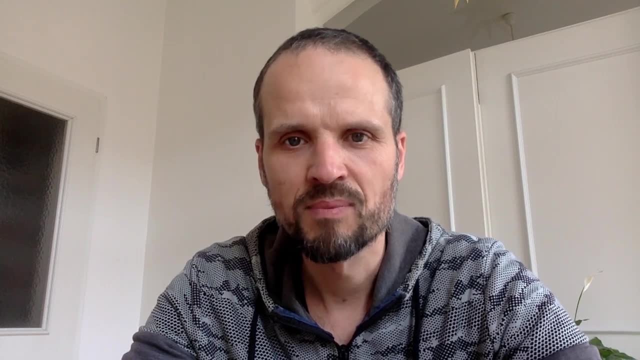 aleph zero. many countable models. Note by our assumption that the signature is countable. This is the maximum possible. There are only 2 to the aleph zero. many countable structures with a countable signature. I will now mention some famous results in this context and a. 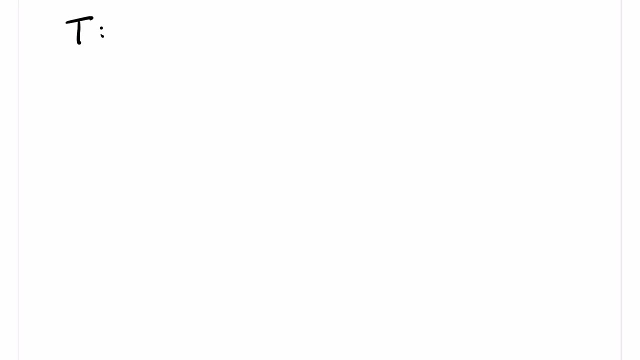 famous open research problem. Let T be a complete theory over a countable signature. Watt's theorem states that T can't have exactly 2 countable models up to isomorphism. Exactly 1 is possible, as we have seen, but not 2. Morley proved that if T has infinitely many, 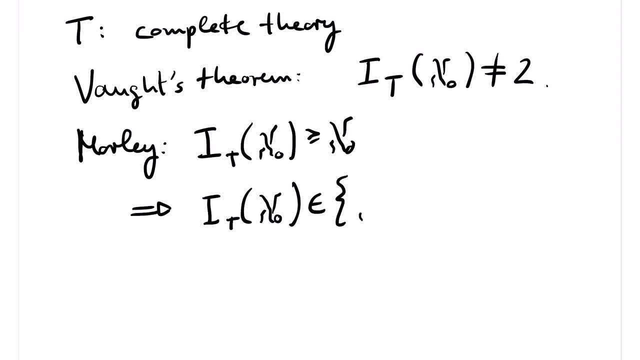 countable models, then there are either countably many models or continuum many, or perhaps aleph 1, many countable models. Aleph 1 is the smallest uncountable cardinal and if the continuum hypothesis does not hold, then this is a different cardinal than 2 to the. 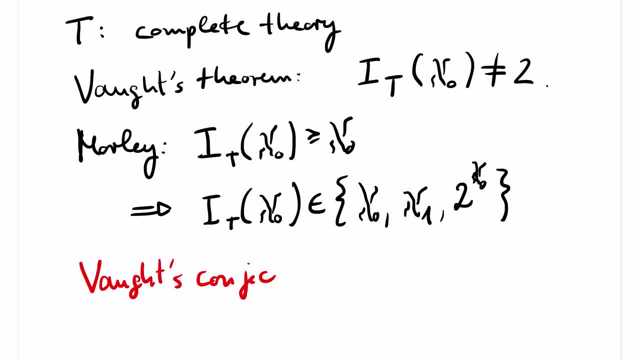 aleph zero. Now Watt's conjecture, which is still open, states that we can remove aleph 1 from the statement. So it states that as soon as we have uncountably many countable models, we have continuum many countable models. 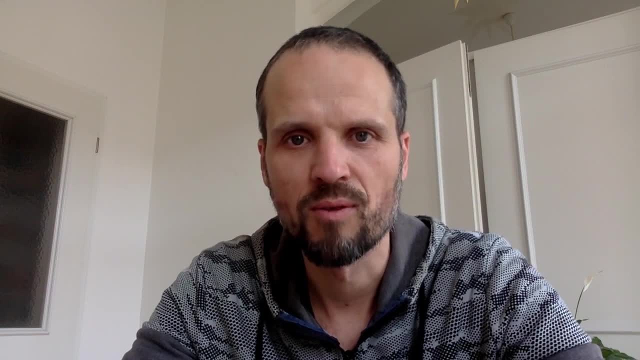 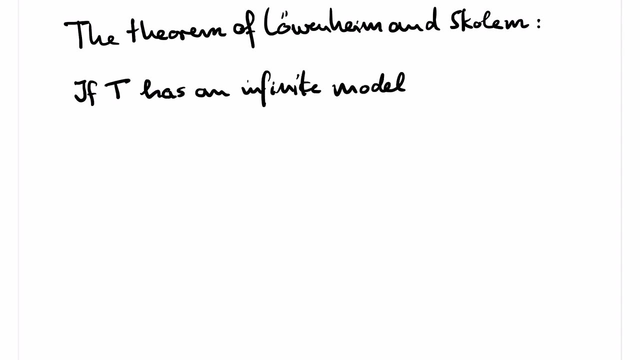 The first that we will prove in this course is the theorem of Löwenheim and Skolem. The theorem of Löwenheim and Skolem states that if t has an infinite model, then it also has a model in every infinite cardinality. Note that this statement has implicitly two parts. There is Löwenheim-Skolem. 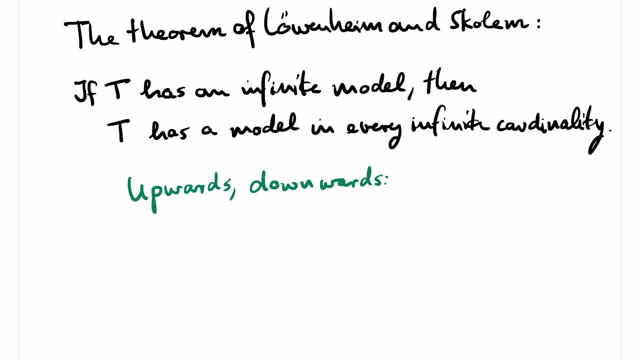 upwards and Löwenheim-Skolem downwards. Let me explain. We have the well-ordered cardinals RLF0, RLF1 and so on. Now suppose we are given some infinite model of t, of some cardinality. Then we have the task to construct larger models of t and we have the task to construct smaller. 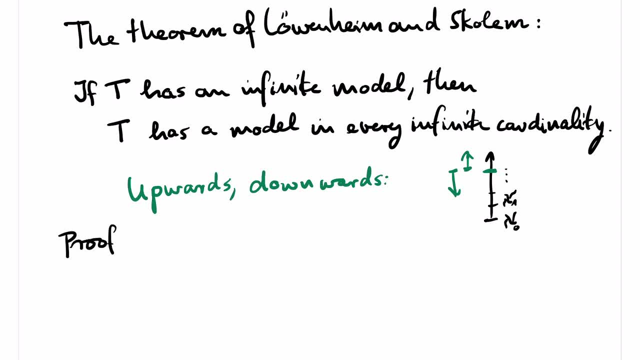 models in order to prove the theorem of Löwenheim and Skolem. To do this, we need to apply a couple of fundamental techniques in model theory that we need all the time. later, In particular, we will introduce LF0.. We also need the compactness theorem of first-order logic, If you haven't encountered 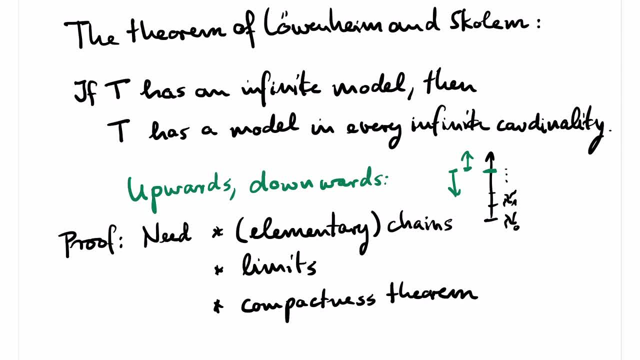 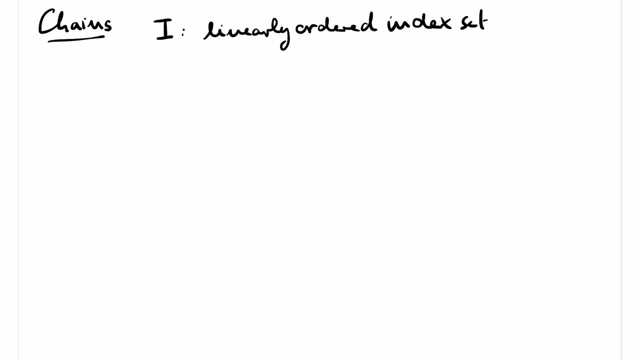 the compactness theorem before. don't worry, we will also prove the compactness theorem. Our proof of the compactness theorem is based on the beautiful ultra product construction. To define chains we need a linearly ordered index, set i and the sequence of structures with the same sequence. 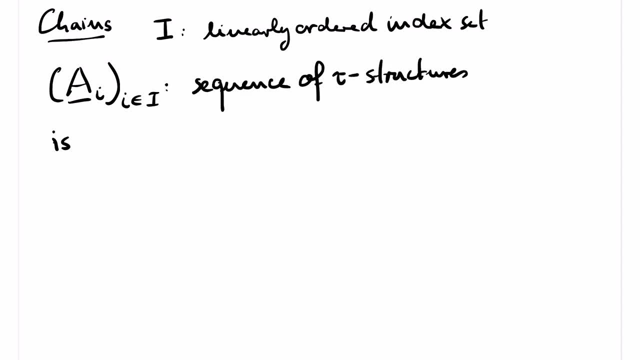 For example, if i is smaller than j, a, i is a sub-structure of a- j, so the chain in fact looks like an onion. A union of a chain is the whole thing viewed as a structure. Formally it is the structure with the. 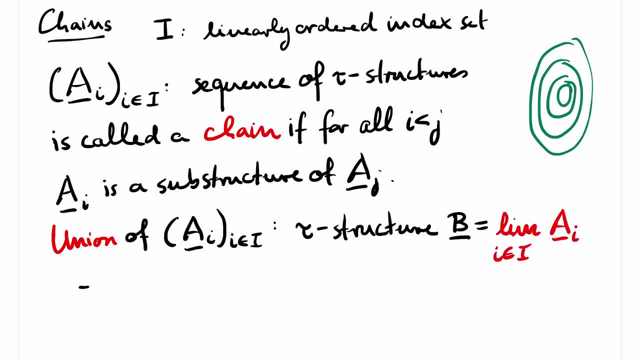 same signature as the structures in the chain whose domain is the union of all the domains of the structures in the chain And where a tuple is in one of the relations. if, for some index i, the tuple is in the corresponding relation in the i-th structure of the chain. 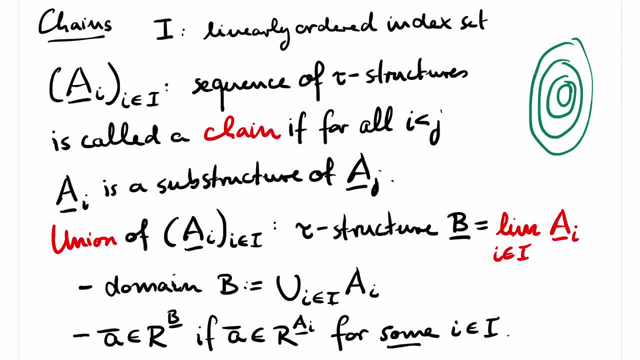 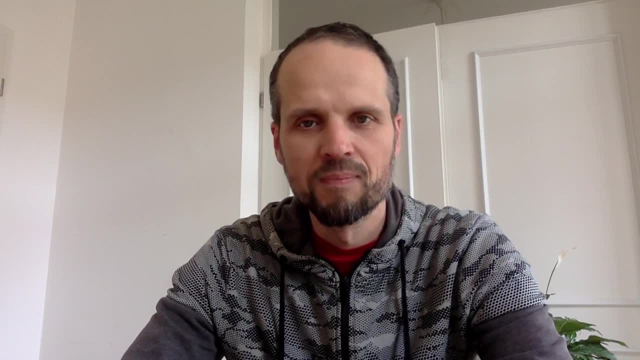 Note that if the index set is well ordered, then this is equivalent to saying that the tuple is in the relation for all but finitely many indices. If the signature contains function symbols, The definition of limits is similar. We have to look at an example. 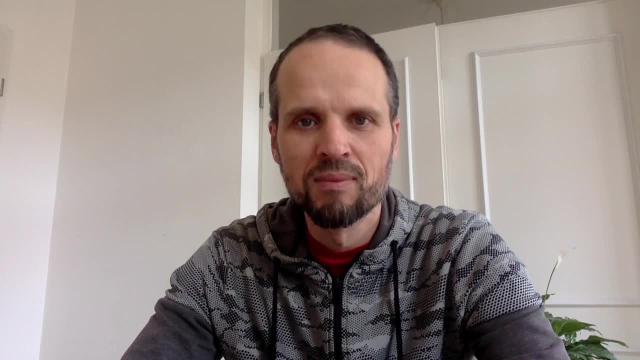 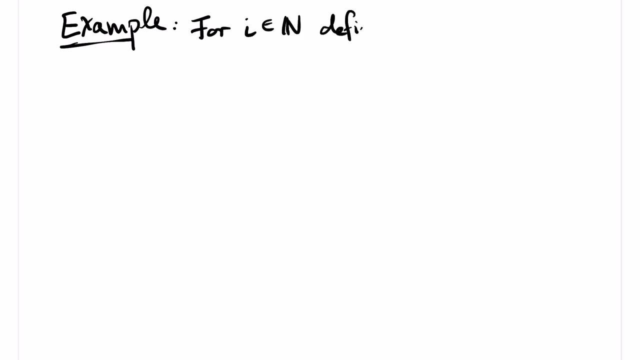 The example I will show you is quite instructive. It will show up two times in this video. Let a i be the structure with domain minus i, minus i plus one, minus i plus two, and so on. so all integers that are larger than minus i minus i included. 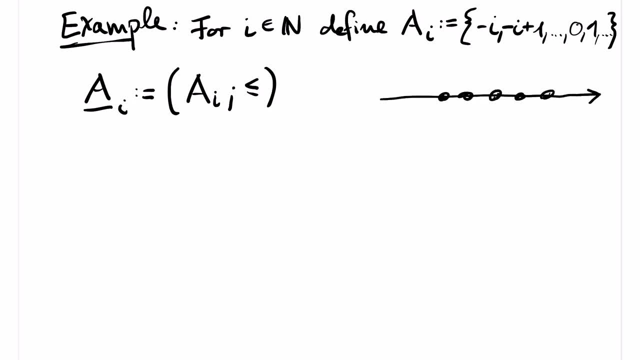 There is only one binary relation in our structure, namely the usual ordering on the integers. Note that for every i, the first-order theory of a i equals the first-order theory of a zero, So all the structures in the chain satisfy exactly the same first-order sentences. 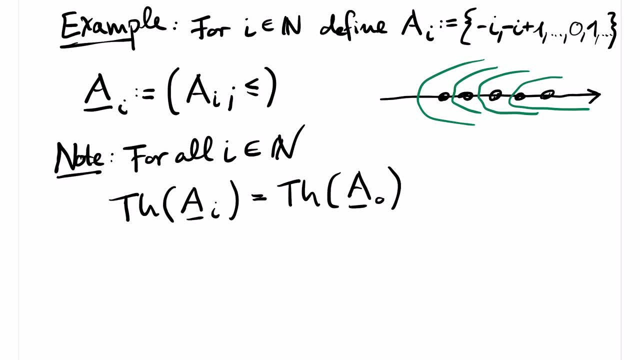 The reason is that all the structures are even isomorphic. However, the first-order theory of the limit of the chain has a different first-order theory. The reason is that in the limit there is no smallest element which is a property that can be expressed by a first-order sentence. 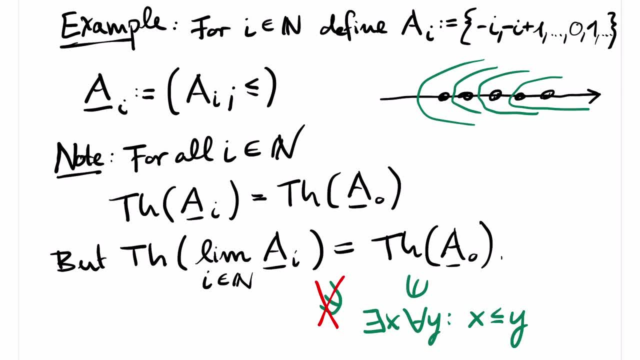 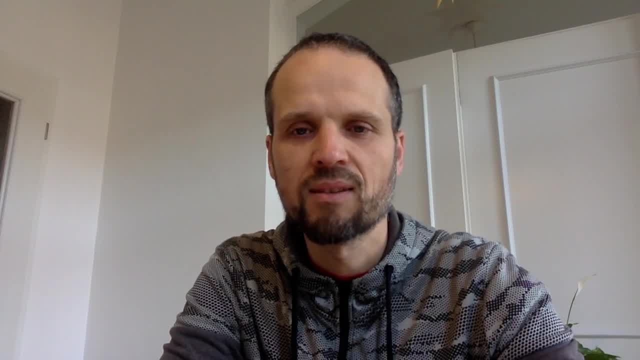 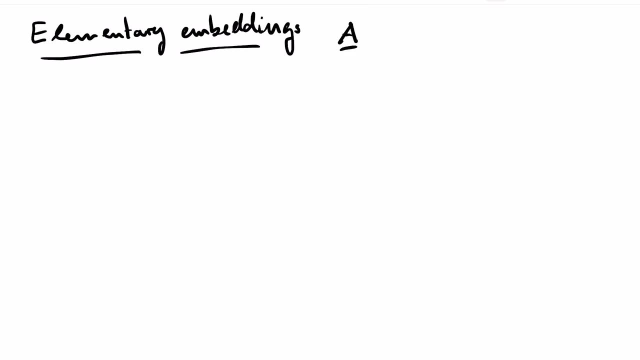 So for this chain, in the transition to the limit, we change the first-order theory. We would like to work with chains that are better behaved in this respect. This is the motivation for the definition of elementary chains. First, we need to define elementary embeddings. 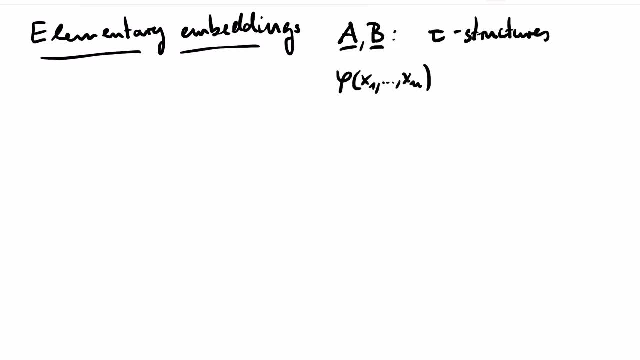 Let a and b be structures with the same signature and let phi be a first-order formula with three variables: x1 up to xn. We say that a function from the domain of a to the domain of b preserves phi If all elements a1 up to a, n of a. if these elements satisfy phi in a, then the image. 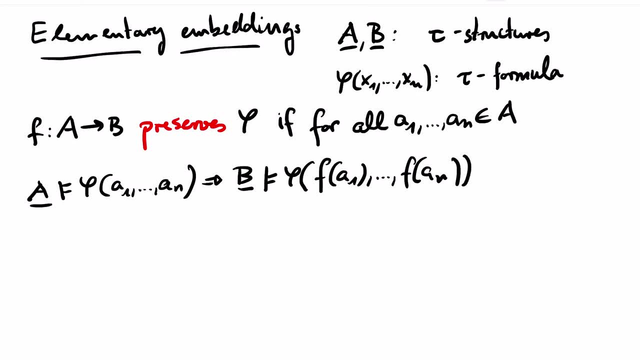 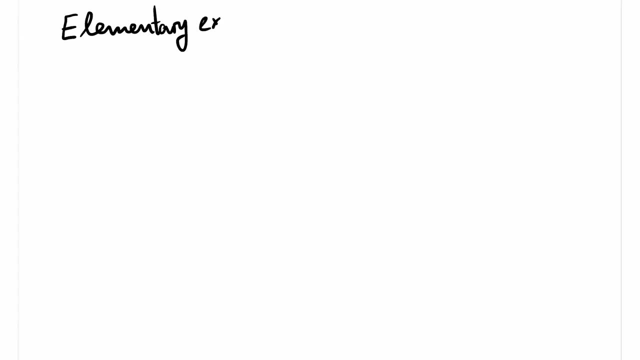 of these elements under f satisfies phi in b. f is called elementary if it preserves all first-order formulas. Let a and b be structures with the same signature and let phi be a first-order formula with three variables: x1 up to xn. We already know what substructures and extensions are. 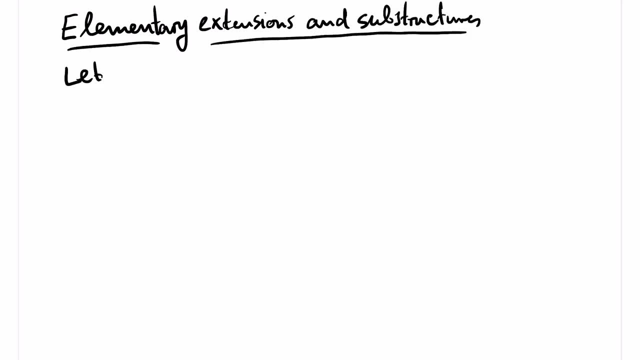 Now we define elementary substructures and elementary extensions. Suppose that a is a substructure of b. If the identity map from a to b is elementary, we write a, break b and call a an elementary substructure of b and b an elementary extension of a. 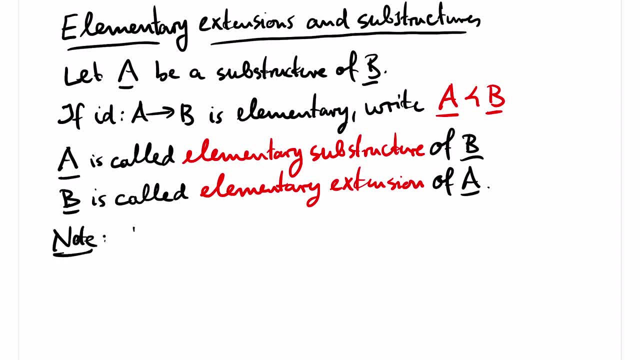 that if a is an elementary substructure of b, then a and b in particular have the same first order theory. the converse need not be true. in our previous example we had that a0 and a1 have the same first order theory, but a0 is not an elementary substructure of a1. to see this, 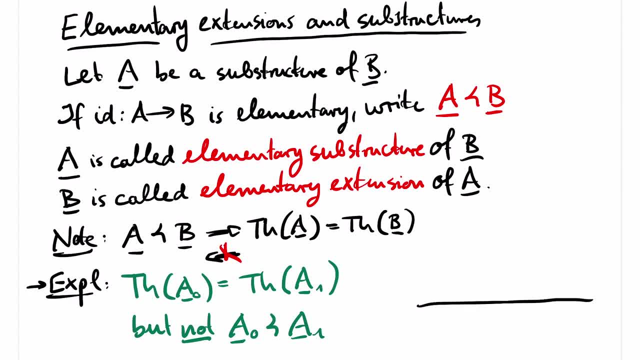 consider the formula phi with one free variable, x, which states that x is a smallest element. this formula holds for 0 in the structure a0, but it does not hold in a1. so the identity map from a0 to a1 does not preserve this formula, so the identity map is: 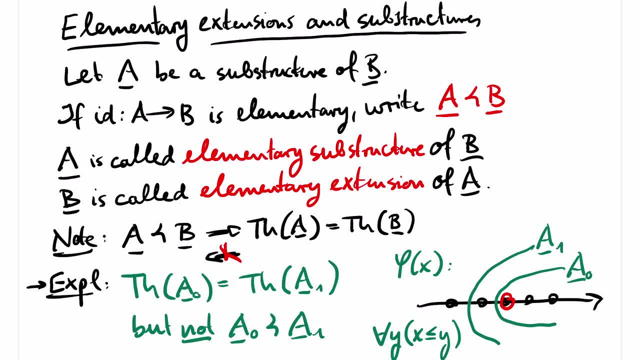 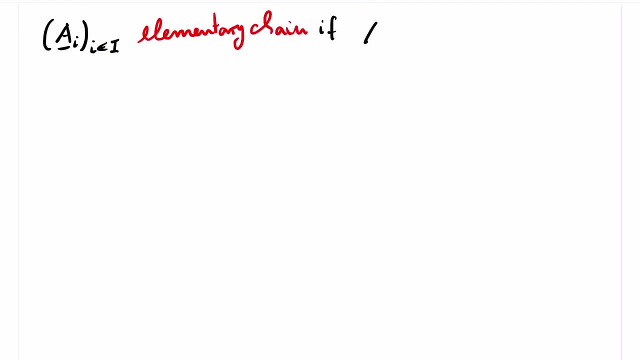 an embedding but not an elementary embedding. a chain a i is called an elementary chain if a i is an elementary substructure of a j for all i smaller j. tarski's elementary chain lemma, or sometimes also called tarski-watt lemma, states that for elementary chains the transition to the limit is smooth. 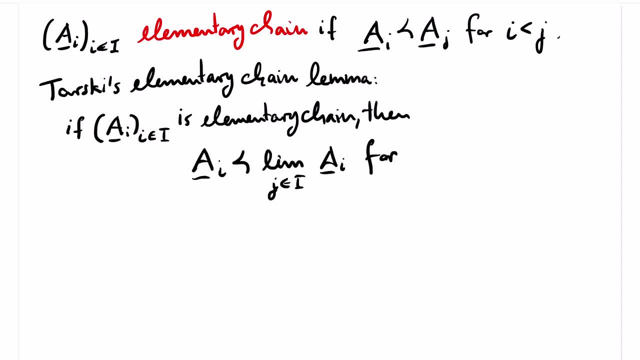 in the sense that every a, i is an elementary substructure of the limit. in particular, the limit will have the same first order theory as the structures of the elementary chain. let's sketch the proof of this lemma. it is by induction over the shape of first order formulas for atomic first order formulas. 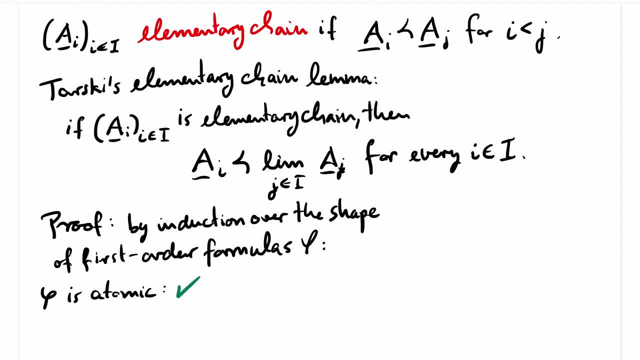 this is immediate already from the fact that a? i is a substructure of the limit. if phi is of the老師 eAD-b Miraet to the matrix a0 a. a i is an elementary substructure of the limit sobre a e calculation that f action is a sum of the structure. eo e is a substructure. eo e grace by time. 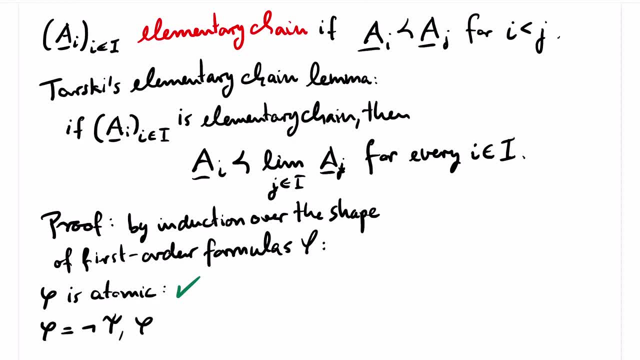 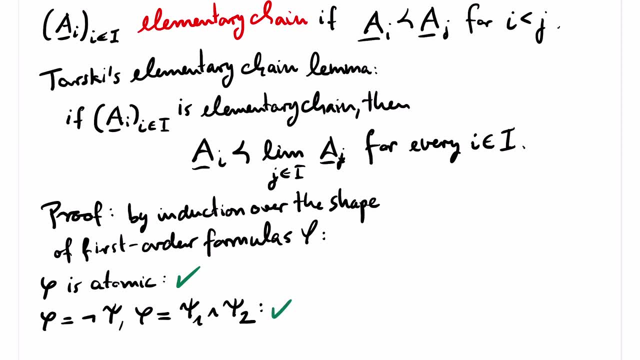 is of the form not psi, or if phi is of the form psi1 and psi2, then the statement follows immediately from the inductive assumption. It is really the existential quantifier that is interesting here. Let's assume that phi is of the form exists and x psi If phi holds. 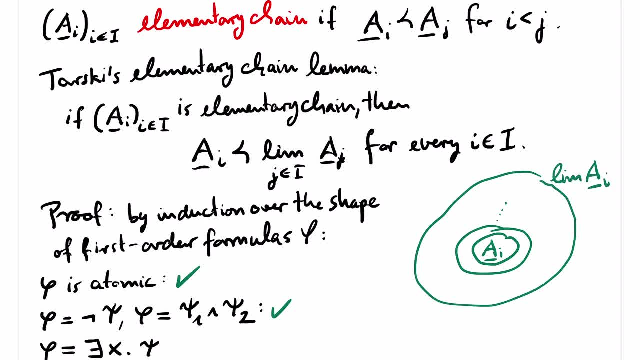 in ai, then it clearly holds in the limit as well, because the witness for x in ai is also an element of the limit. so this direction is trivial. For the other direction, suppose phi holds in the limit. Now the witness for x might not be an element of ai. However. 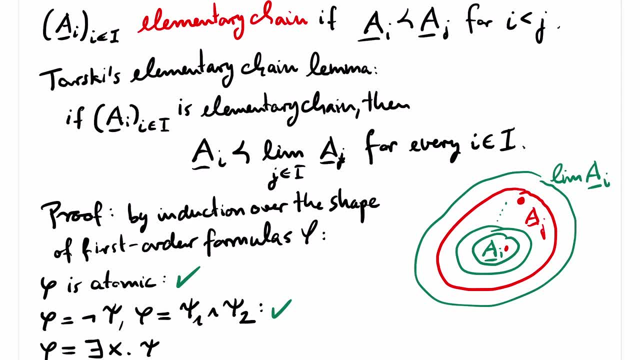 the witness is an element of aj. for some j by the definition of the limit, aj does satisfy phi, But aj is an elementary extension of ai, so ai also satisfies phi. And this concludes the proof In the proof of the downwards Leuvenheim-Scholem. 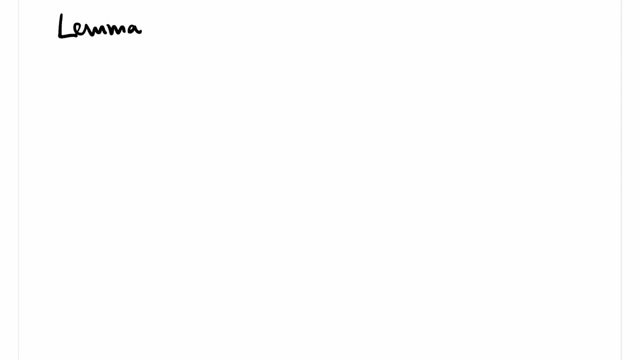 theorem. we need a lemma that is somehow similar. It is called Tarski's test. It is a test whether a certain subset of the domain of a structure is the domain of an elementary substructure. So we have a structure B And a subset of the domain of B. The lemma says that A is the domain of an elementary. 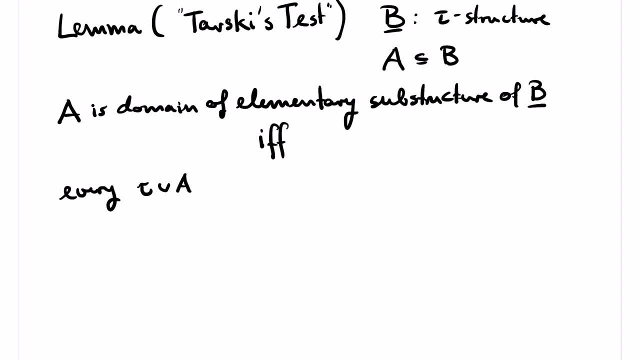 substructure of B, if, and only if, every formula phi that might also involve constants from A and is satisfiable in the expansion of B by those constants can also be satisfied by an element of A. So slowly again with a picture: We have B and we have the subset A. 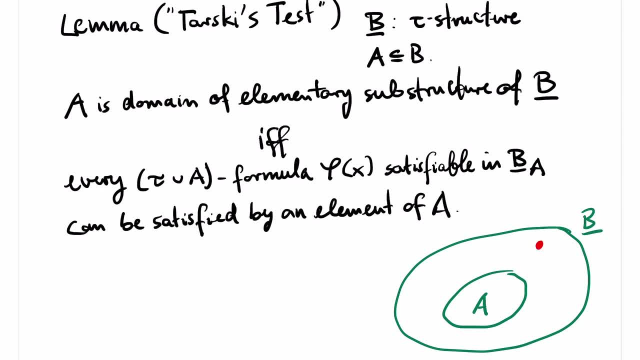 And we require that if some formula is satisfiable in B, then it is already satisfiable in A. But the important thing is that our formula might talk about all the elements of A, because we have expanded the structures so that they have constants for all elements of A. 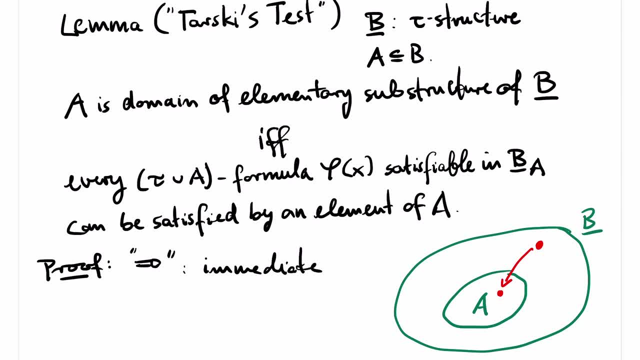 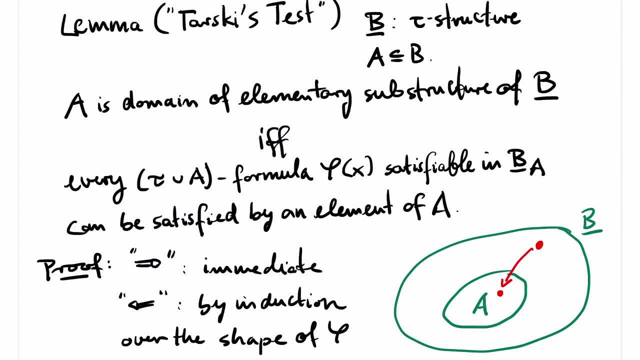 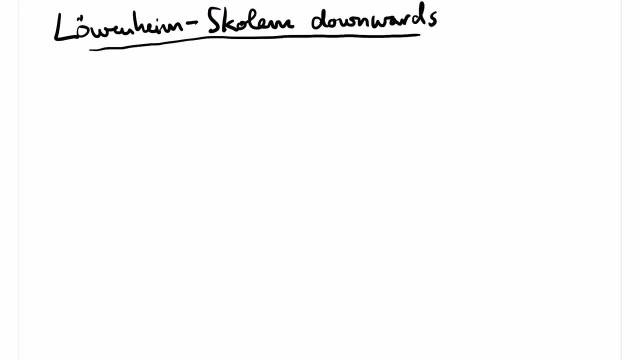 It request original induction over the shape of first-order formulas, and we leave it to the audience. Finally, we can prove Louvain-Hijms-Schulheim downwards. Let B be a structure and let S be a subset of the domain of B. 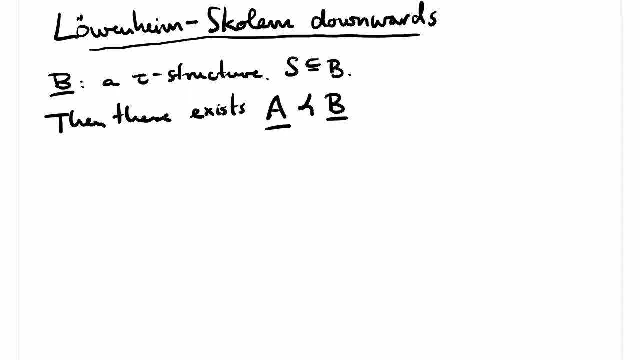 We will show that B has an elementary substructure, A, whose domain contains S and such that it has cardinality, at most the size of S, at least countable. So if s is finite, then a is still allowed to be infinite. In our proof we construct a chain. We start with s and define the elements of the chain. 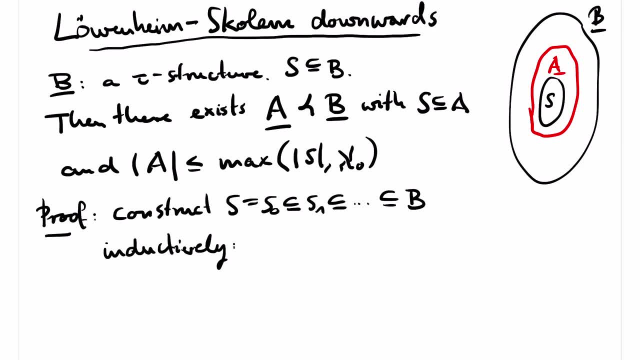 as 1, as 2 and so on. inductively Suppose that s is already defined. To define s, we look at all formulas phi with only one free variable, x, which are satisfiable in b. The formula might contain constants from s. 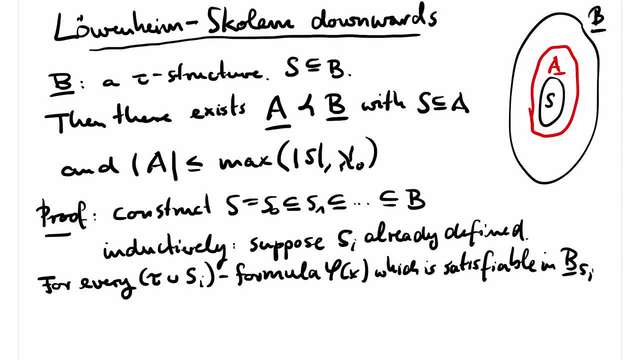 Since the formula is satisfiable in b, we can choose a witness for x in b. Let's call the witness a sub phi. b satisfies phi of a sub phi. And now s contains s, together with all these witnesses for all formulas phi, And in this way we get the formula. 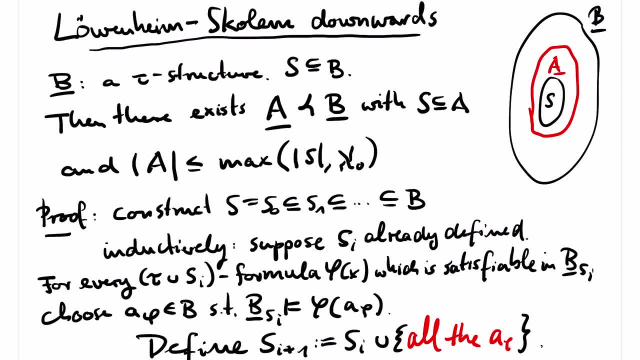 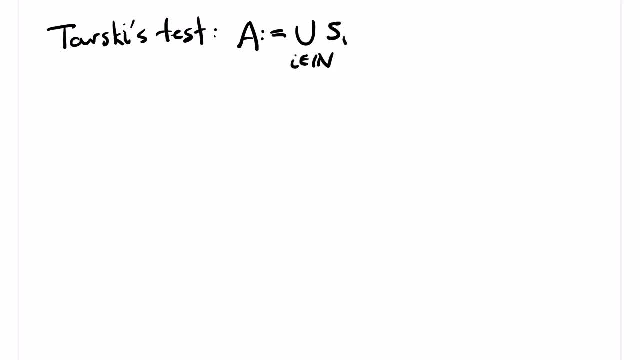 We repeat, constructing our chain. My first claim is that the union a of all the s, i is an elementary substructure of b, And this is precisely the purpose of Tusky's test. So let's have a look at an illustration. We have a, b, We have the subset. 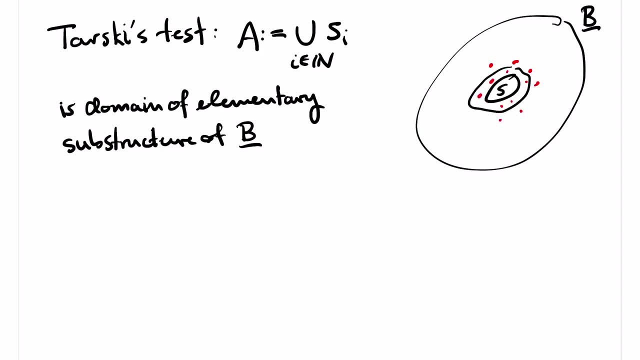 s Now we construct our onion by including witnesses for formulas. We have to verify that the union a of the sets we have constructed satisfies the assumptions from Tusky's test. So we have some formula which might use constants from a and which is satisfiable in b. 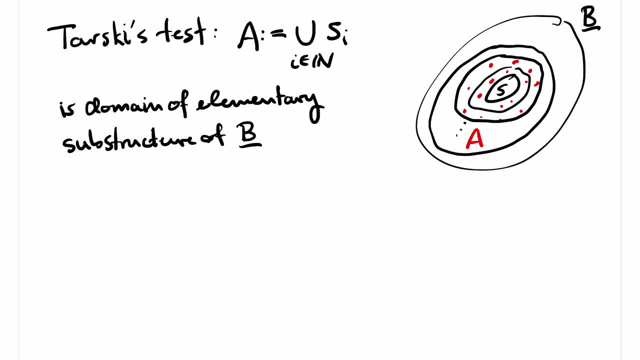 Then there will be a layer in our onion that contains all the finitely many constants that we use in this formula, And this means that on the next layer of the onion we have added a witness for this formula, So the onion contains the witness. This is precisely what we need for Tusky's test. 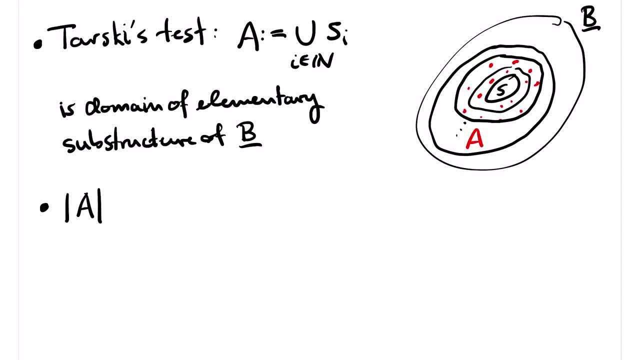 My next claim is that the union a of all the s, i has at most the cardinality of s, unless s is finite, in which case a is countable. This is an easy calculation: Each layer has at least the size of s. 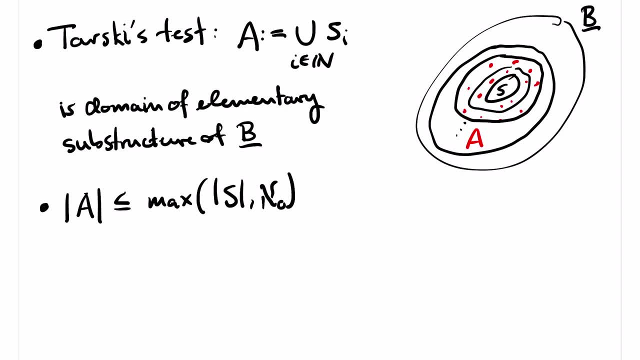 and then we prove by induction that each layer has a size at most max of the size of s and aleph zero. this is because of our assumption that the signature is countable, because then there are only that many formulas. so we added only that many witnesses and we have countably many layers. 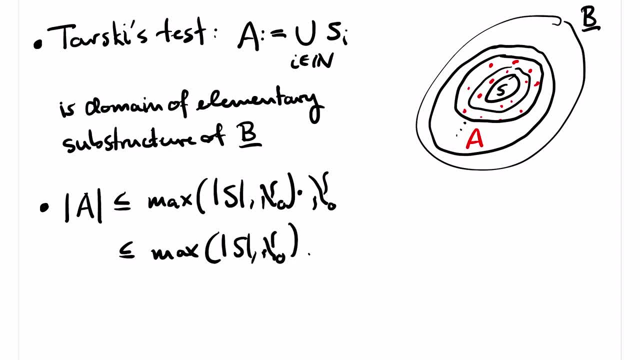 but countable times. kappa equals kappa for every cardinal kappa and this shows the claim. the upwards lorvenheim scholen theorem is an easy consequence of the compactness theorem, so we will defer this to the next video about compactness. i will explain the idea of this. 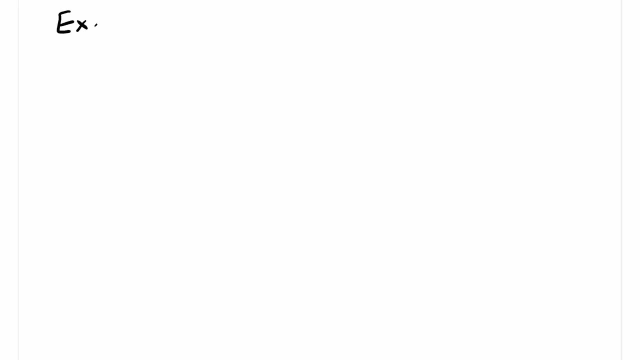 chain construction. again with an example, we consider the structure of the linearly ordered real numbers. this structure has cardinality two to the r of zero. we would like to construct a countable model with the same first-order theory. in this example you might see the countable model. 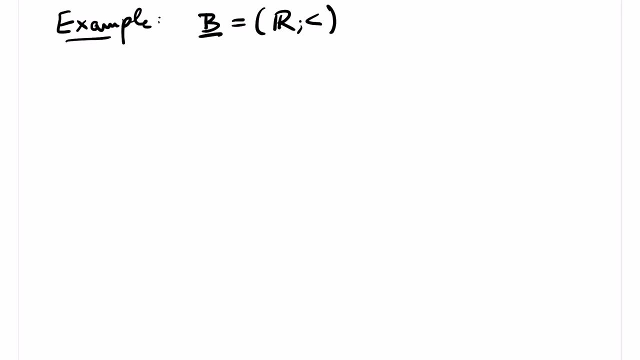 immediately. but the point here is that I would like to illustrate the idea of the proof of the downwards-Leuvenheim-Scholem theorem with this example. We first fix arbitrarily some countable subset. Suppose we start with z, the integers Now. 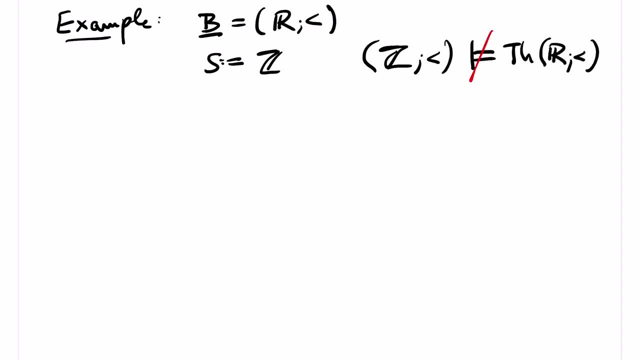 the integers do not have the same first-order theory as the reals. with respect to the linear order, For example, the reals are dense while the integers are not, and this is a first-order property. In the first step of the construction, we look at formulas with one free variable. that 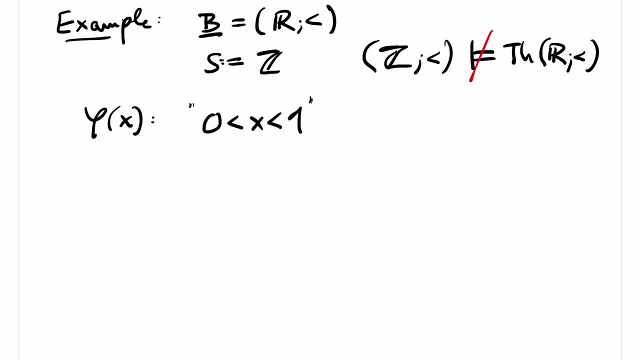 might involve some constants from z. For example, the formula 0 is smaller x and x is smaller 1. This is a formula that is satisfied in b but not in z. So to the next level in the construction we add a witness for x, For example one half. 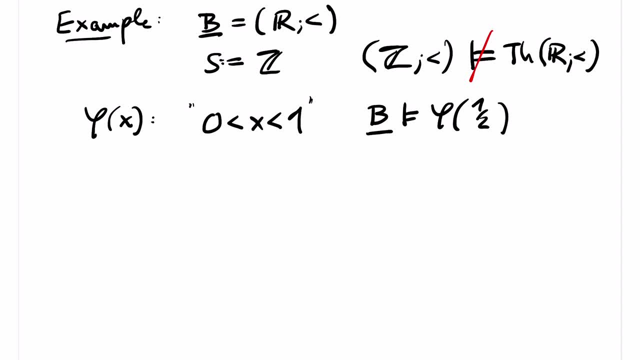 We could have added two thirds doesn't matter, And this we do for all first-order formulas. There are only countably many, since our signature is countable. And then we repeat the entire thing infinitely often And our proof shows that at the end we arrive at a countable elementary substructure of 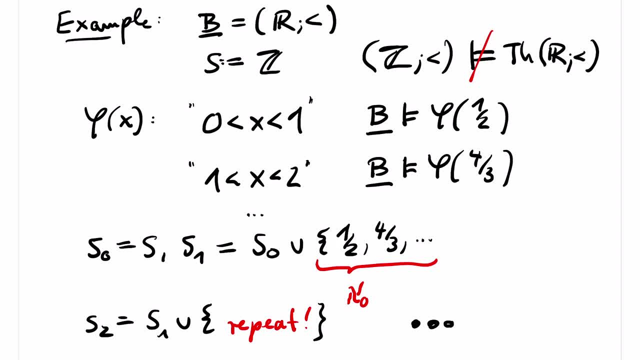 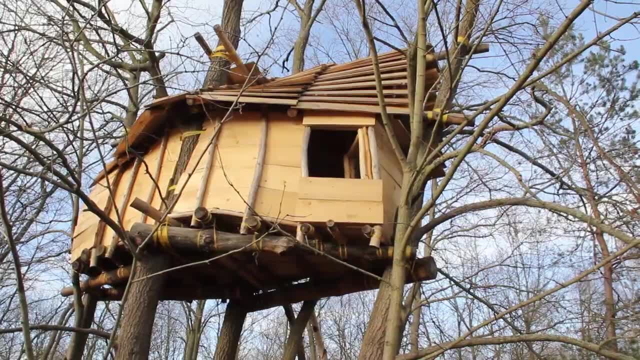 b, which means, in particular, that this substructure has the same first-order theory as the structure we started with. Thank you for watching.